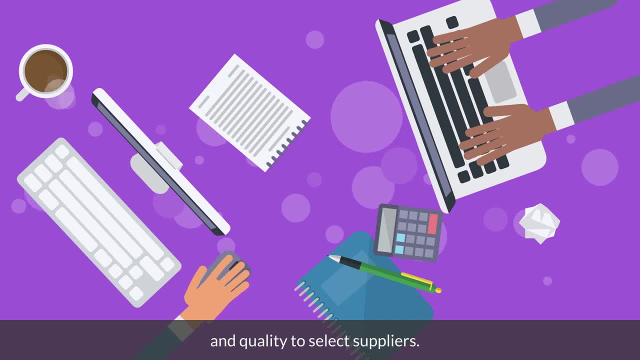 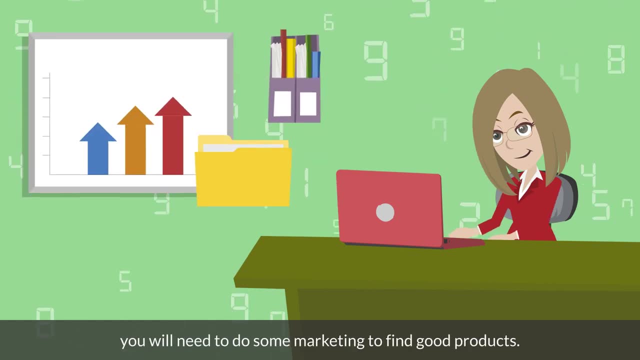 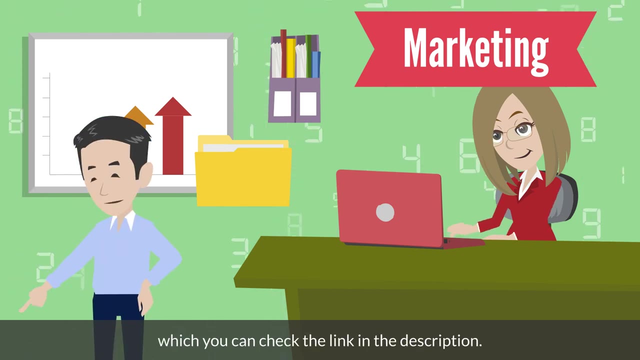 business. you should note price and quality icgov Le�xi local system. However, if you are starting import trade as a new business, you will need to do some marketing to find good products. There is a detailed explanation of marketing in another video which you can check: the link in the description. 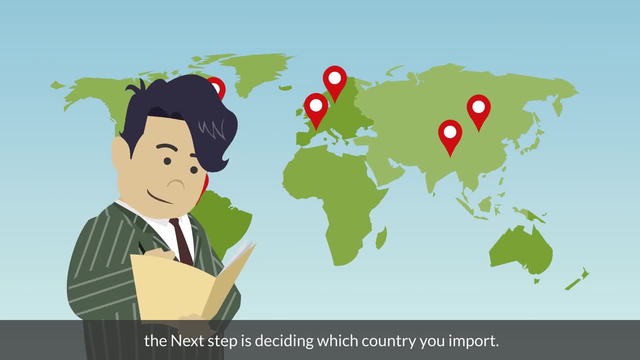 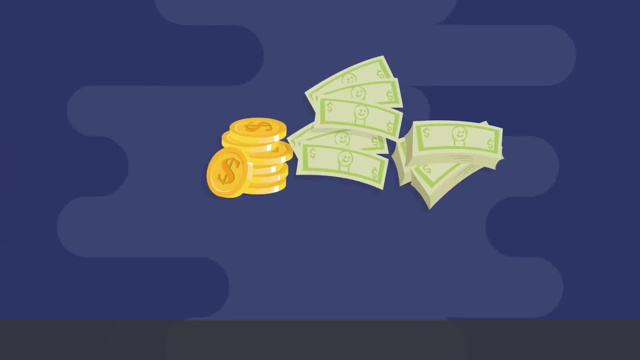 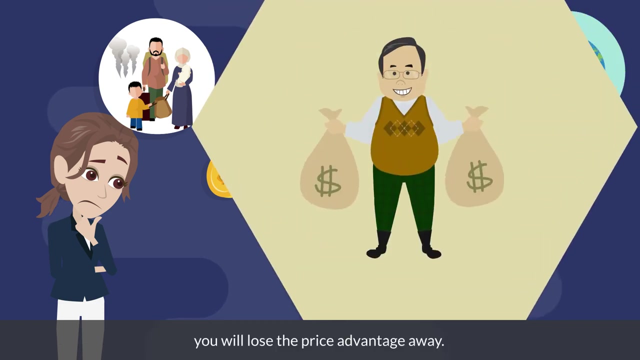 Once you decide on the product you want to import, the next step is deciding which country you import. Choosing a country is very important. Don't just look at the cost of the product. If your country is politically unstable, has no preferential tariffs or is too far from your country, you will lose the price advantage away. 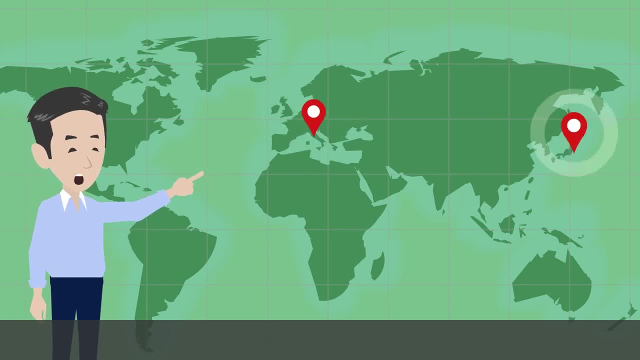 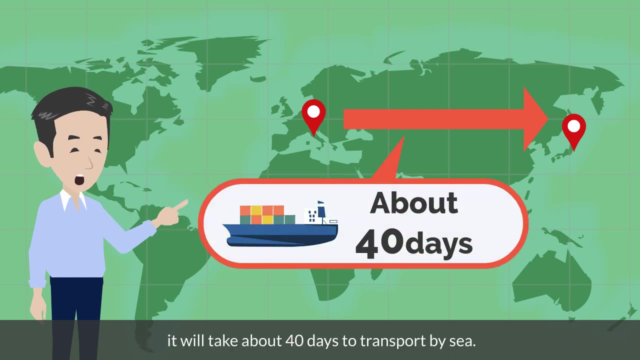 Let's talk a little more about the distance between countries. For example, if you buy products from a European country to Japan, it will take about 40 days to transport by sea. This makes it difficult to adjust stock control and cash flow during the transportation period will be poor. 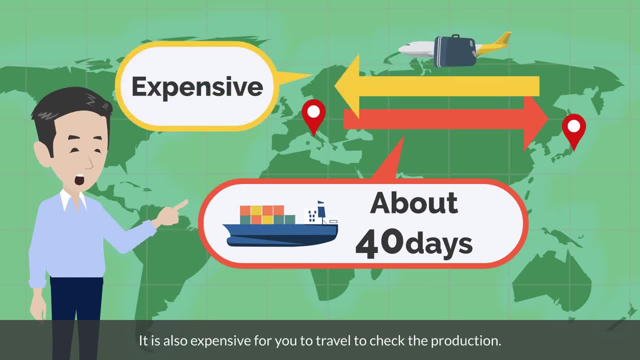 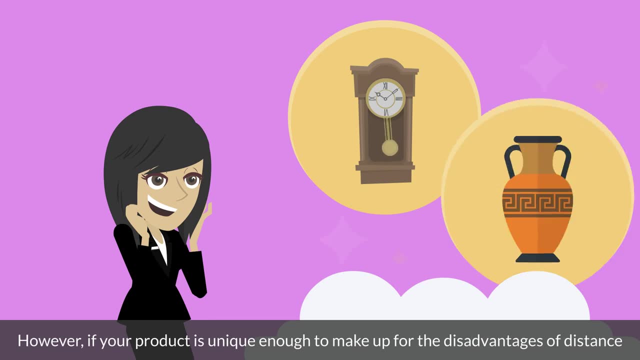 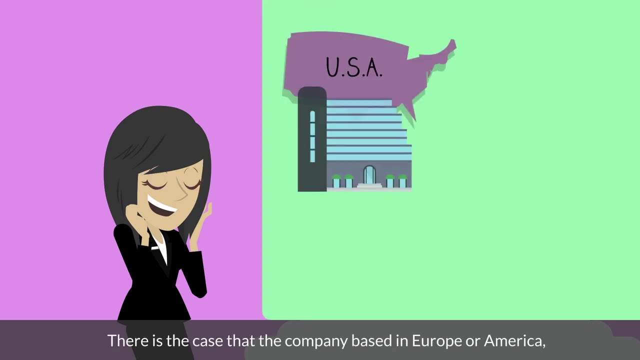 It is also expensive for you to travel to check the production. However, if your product is unique enough to make up for the disadvantages of distance or to differentiate yours from other companies, there will be no problem. There is the case that the company based in Europe or America, but the actual country of production is in China or Southeast Asia. 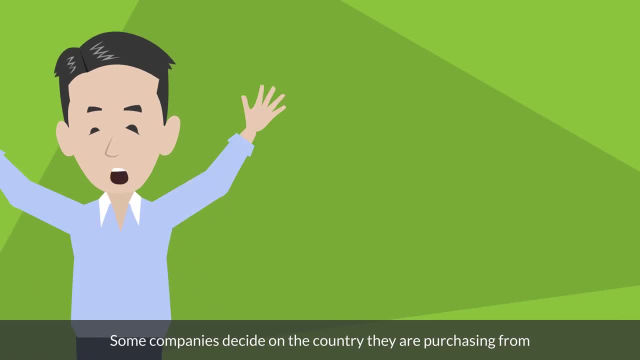 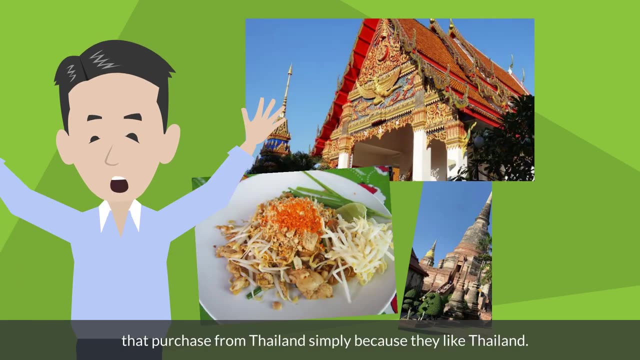 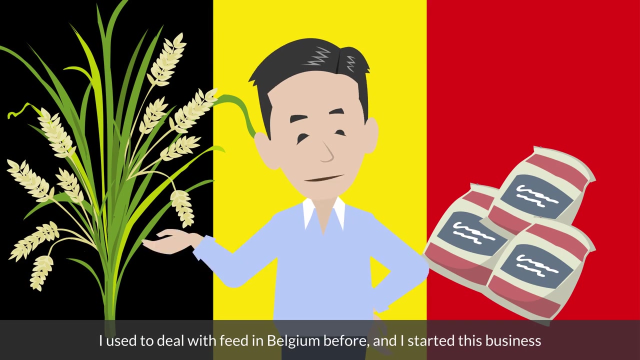 Some companies decide on the country they are purchasing from because they like the country very much. I work in Taiwan And I know several small and medium-sized companies that purchase from Thailand simply because they like Thailand. I used to deal with feed in Belgium before and I started this business because I wanted to drink Belgian beer. 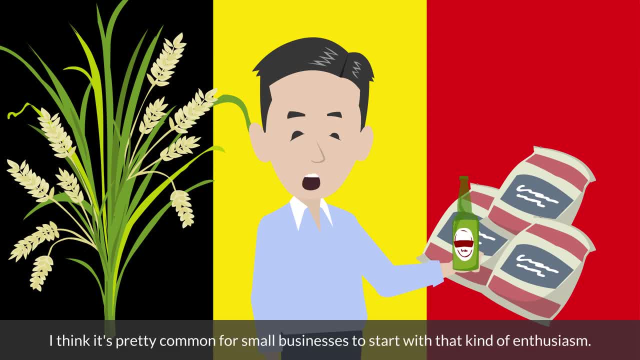 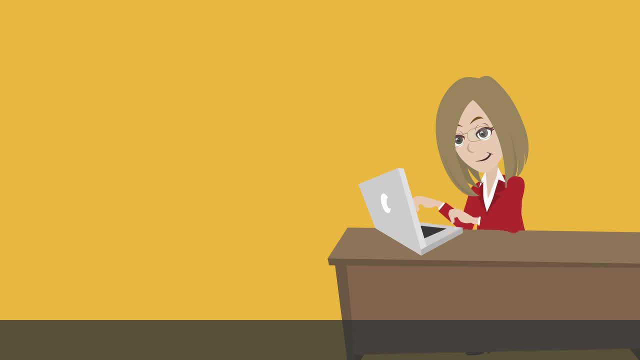 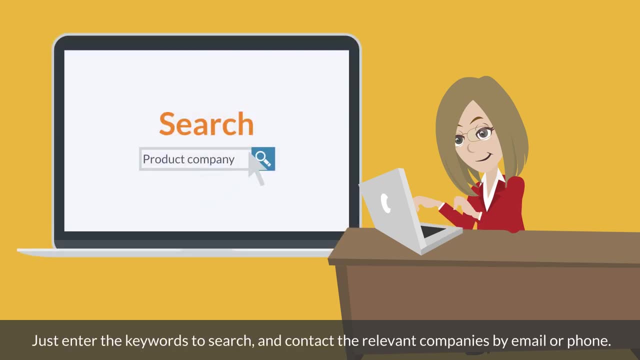 I think it's pretty common for small businesses to start with that kind of enthusiasm. So once you decide on a country to buy, how do you find a company to buy next? Nowadays you can get enough information on the Internet. Just enter the keywords to search and contact the relevant companies by email or phone. 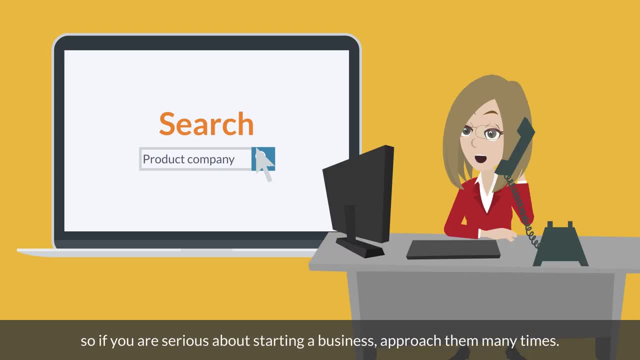 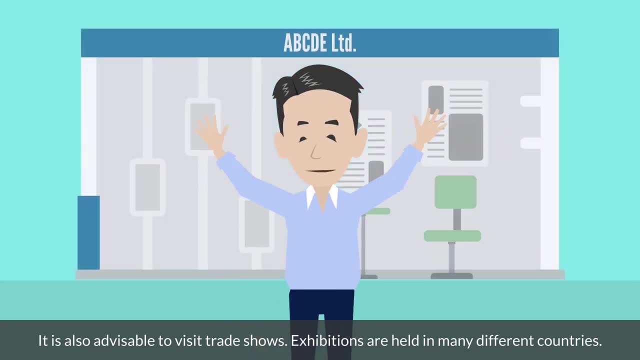 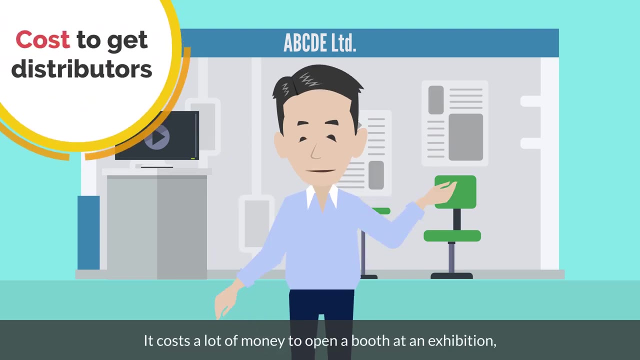 One-time contact is not enough to get a reply, so if you are serious about starting a business, approach them many times. It is also advisable to visit trade shows. Exhibitions are held in many different countries. It costs a lot of money to open a booth at an exhibition, so the suppliers try to find good customers or distributors seriously. 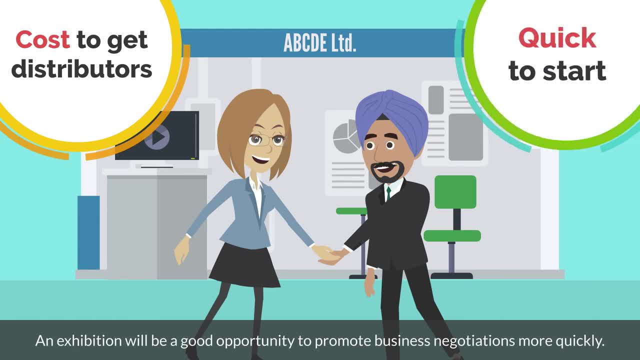 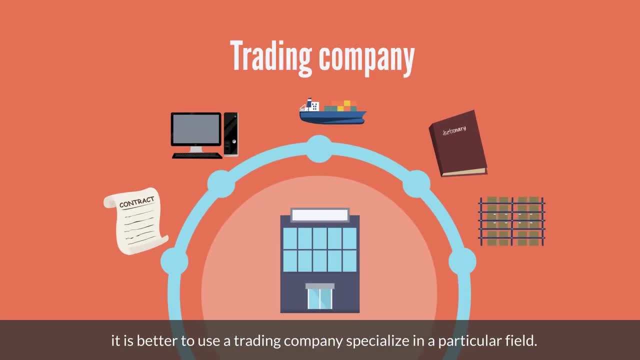 An exhibition will be a good opportunity to promote business negotiations more quickly. If you are worried about the difference in language and business customs, it is better to use a trading company specialized in a particular field. They will import the goods to your home country, so there is some cost as a margin. 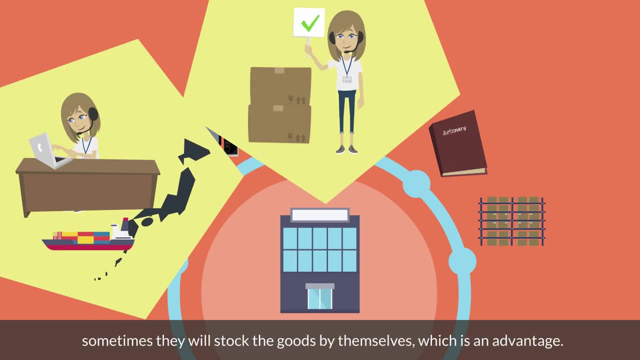 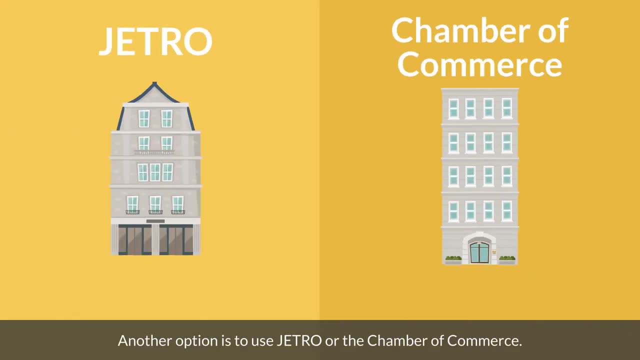 However, you will be able to purchase the small lot and sometimes they will stock the goods by themselves, which is an advantage. Another option is to use Tetra or the Chamber of Commerce. These organizations support companies trying to expand overseas. They provide you with information about local companies and the market situation. 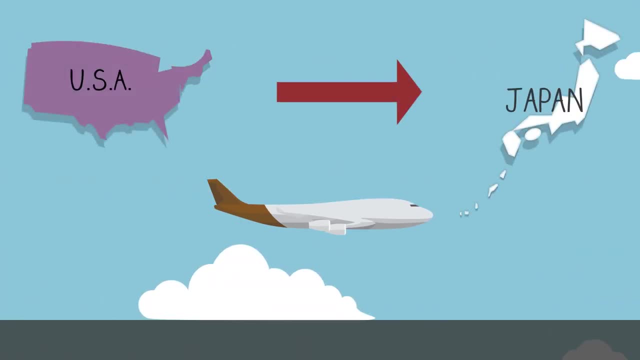 Importing is less difficult than exporting. This is because you are a customer and it is easier to find suppliers than sellers. If you are a beginner in trade, it is better to start with importing than exporting. This is the most important part. 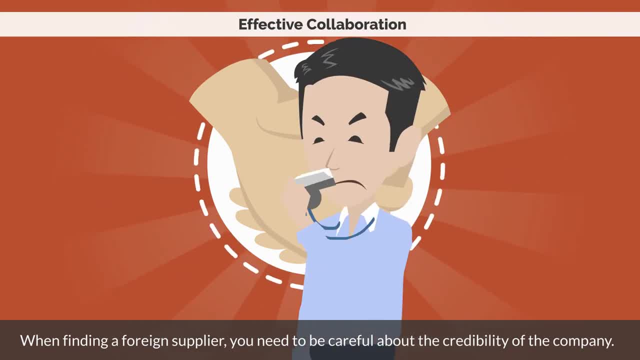 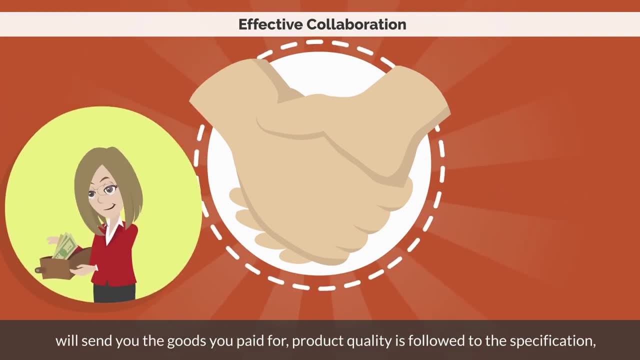 When finding a foreign supplier, you need to be careful about the credibility of the company. In the case of importing, there are some problems whether the company will send you the goods you paid for- product quality is followed to the specification- or they are responsible for the delivery schedule. 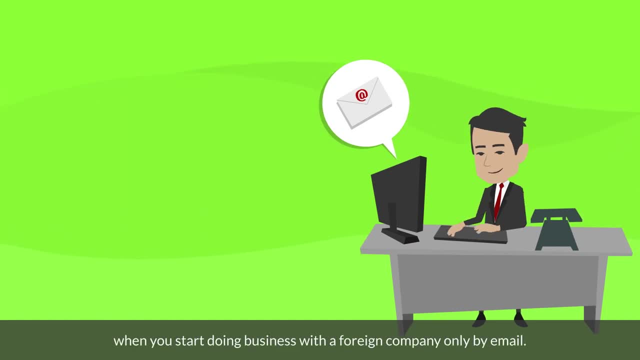 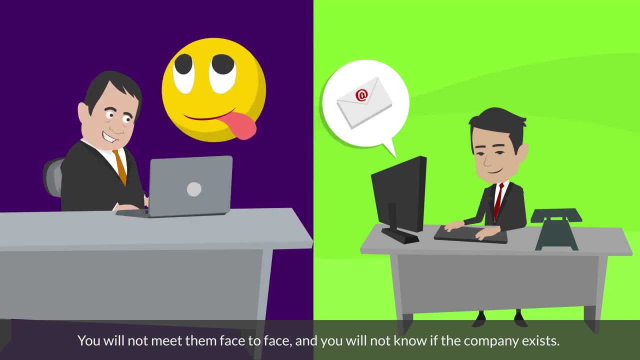 I believe that these credit risks are higher when you start doing business with a foreign company only by email. You will not meet them face to face and you will not know if the company exists. Some companies ask you to send money again because of additional costs or make an unreasonable request. 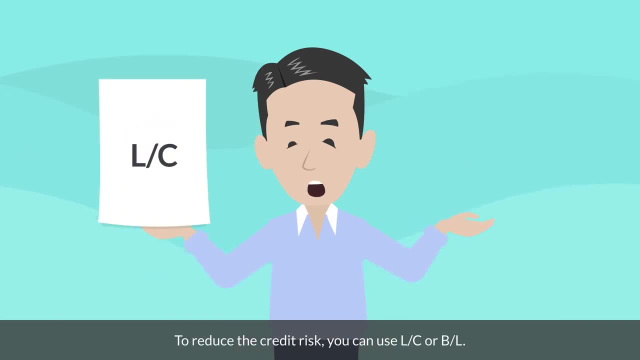 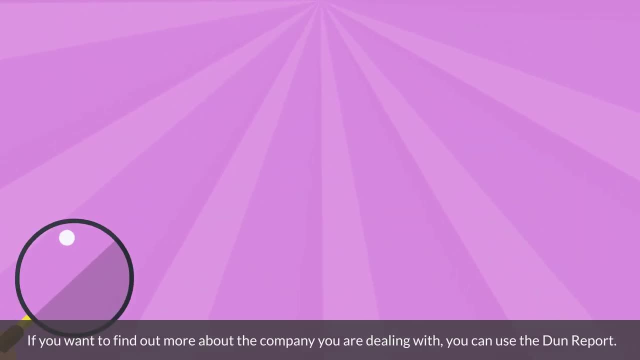 To reduce the credit risk. you can use LC or BL. These are explained in detail in another video which is linked in the description. If you want to find out more about the company you are dealing with, you can use the Dunn Report. 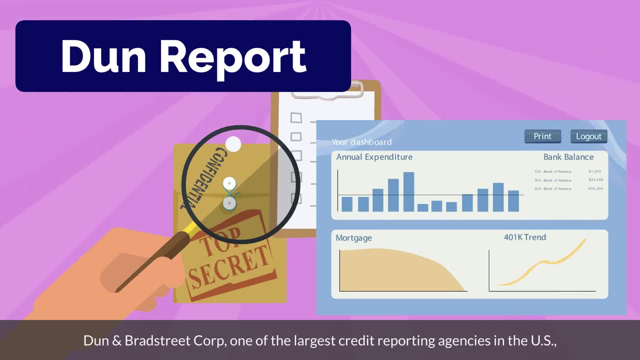 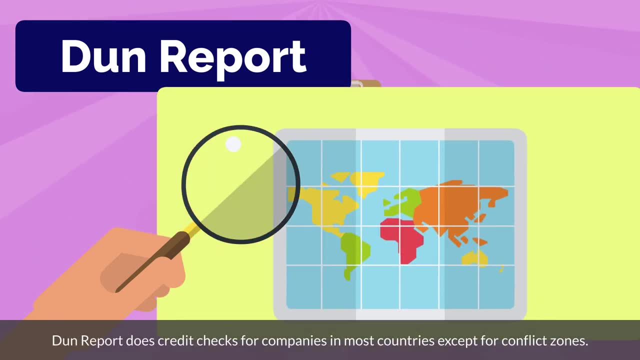 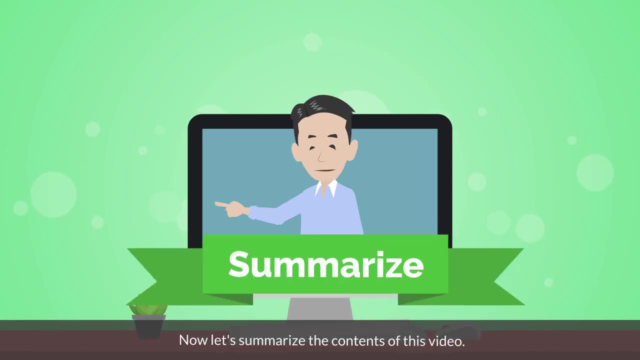 Dunn and Bradstreet Corporation, one of the largest credit reporting agencies in the US, will verify the creditworthiness of your business partners. Dunn Report does credit checks for companies in most countries, except for conflict zones. Now let's summarize the contents of this video. 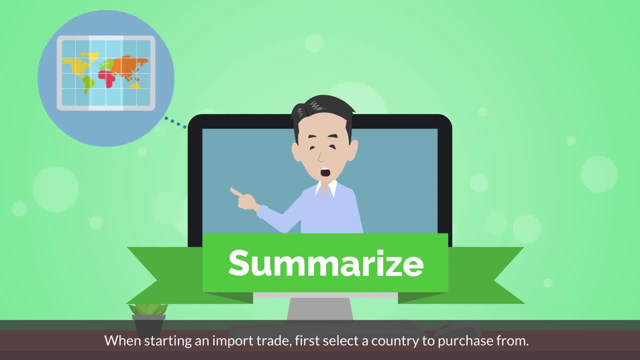 When starting an import trade, first select a country to purchase from. Why do you want to buy from that country? You need to check how much benefit and whether the lead time and cash flow risks are acceptable. Once you decide country, the next step is to find a company to purchase.